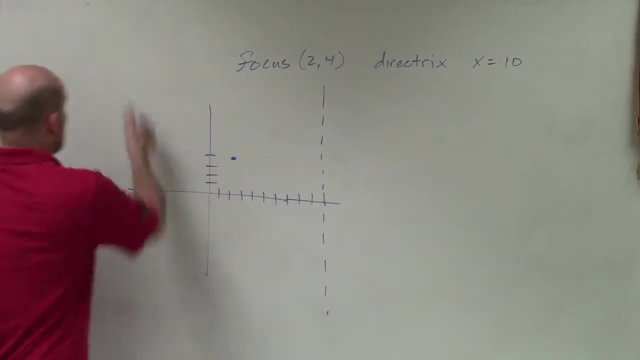 can see, is going to be a distance of 6.. Now remember, when we look at just kind of like the parent graph here of one parabola we have, the focus is always inside of my parabola and the directrix is that exact same distance. If that's p, then this distance is negative. 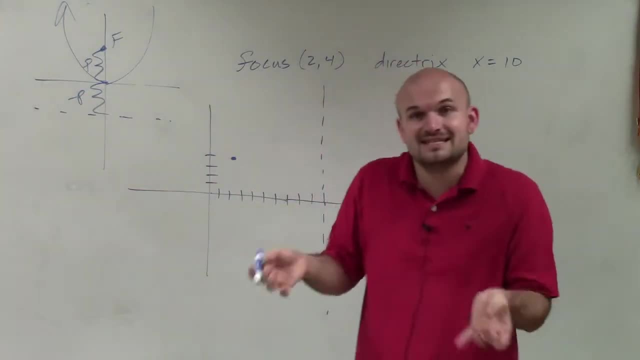 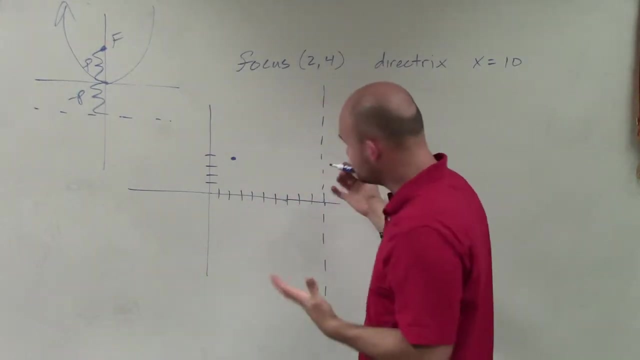 p. So what's important about this is the distances are exactly the same, One's in a positive, one's in a negative direction. But what this will help us out, what it will tell me, is one: my axis of symmetry is going to be perpendicular to my directrix. 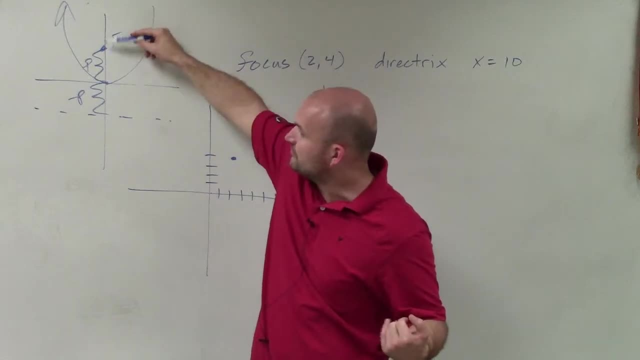 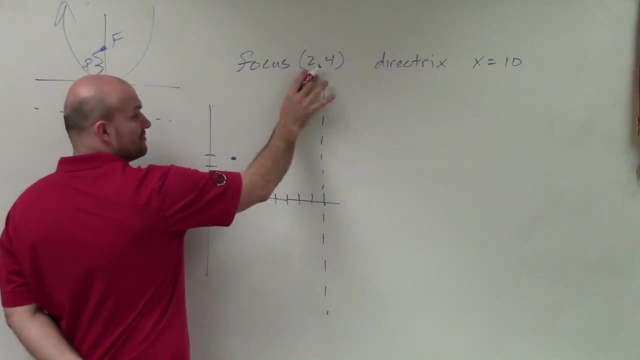 And not only is it going to be perpendicular to my directrix, but it's also going to go through the focus as well as the vertex. So, therefore, I know that my axis of symmetry runs through my point, the focus, which is 2, come 4, as well as going to go through 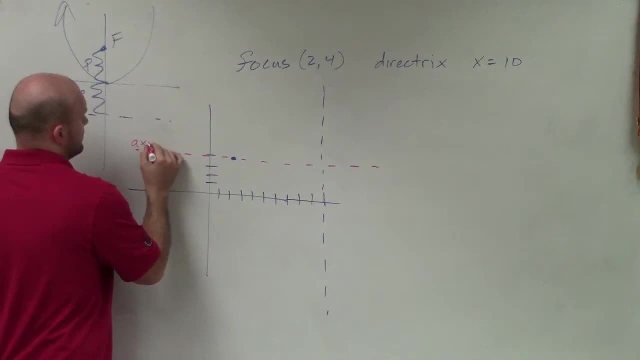 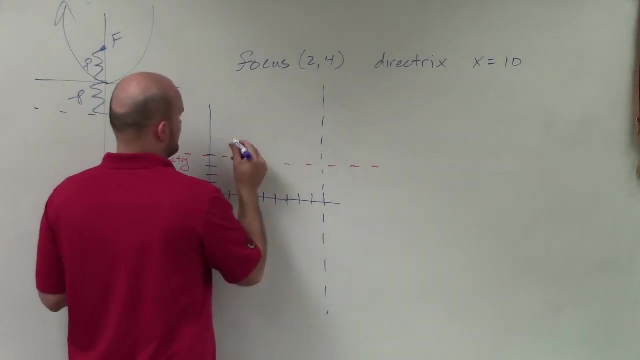 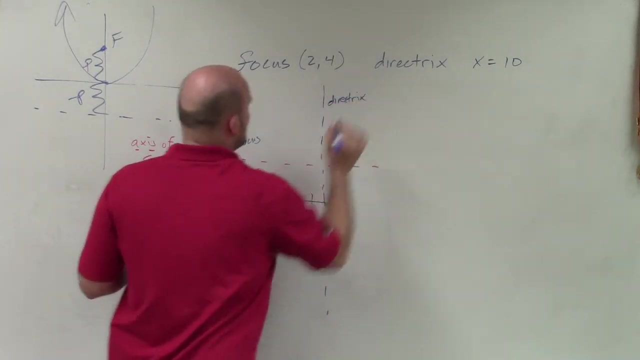 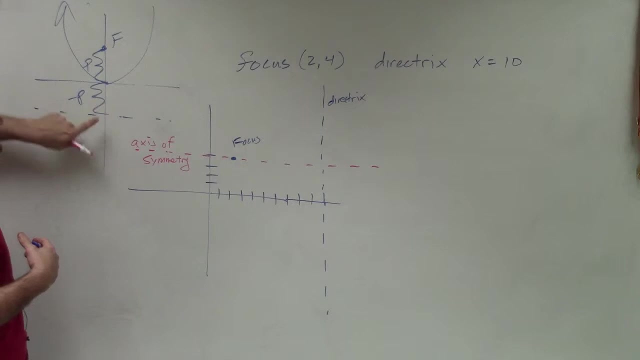 my vertex. So there's my focus and here's my directrix. Okay, so what's important also to notice is that the vertex is also half the distance between my focus and my directrix. You can see, the distance from this vertex is the same to the focus as it is to the directrix. So 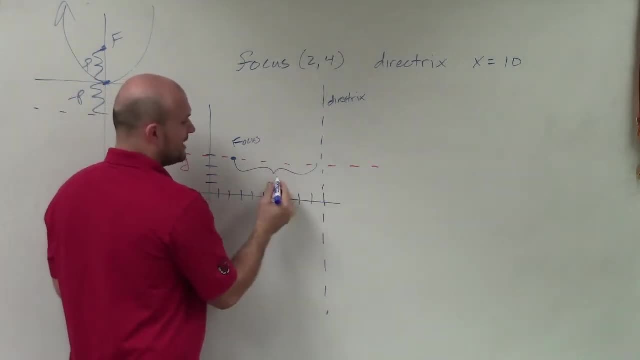 if I have my distance, the total distance here is 6.. Therefore, my vertex then has to be in the middle of that. So it's going to be 3 units to the right of my focus: 1,, 2,, 3, and 3 units to the left. Well, let's hold on. That's it. 2, oh shoot, that's more. 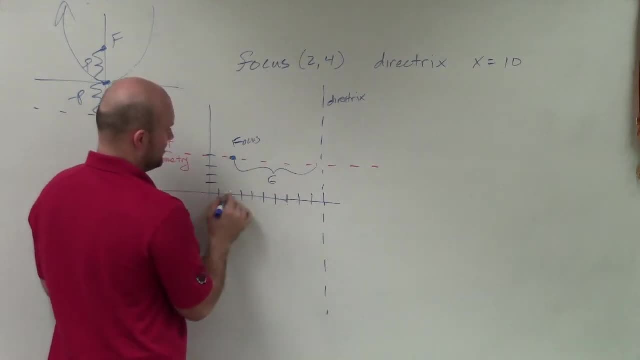 than that, It's 8.. Right, That's it too. I miscounted So 1, 2.. So, therefore, it's going to be 1,, 2,, 3, 4.. So it's going to be 4 units, to the right of my focus, and 4. 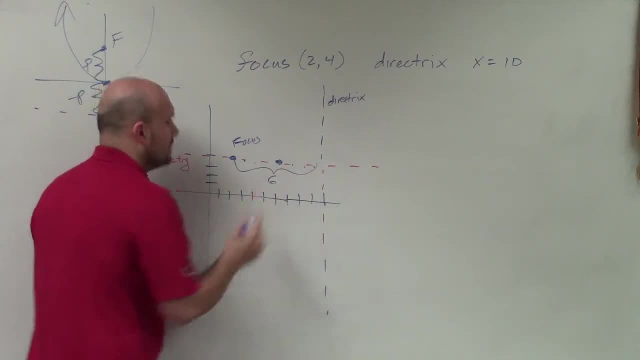 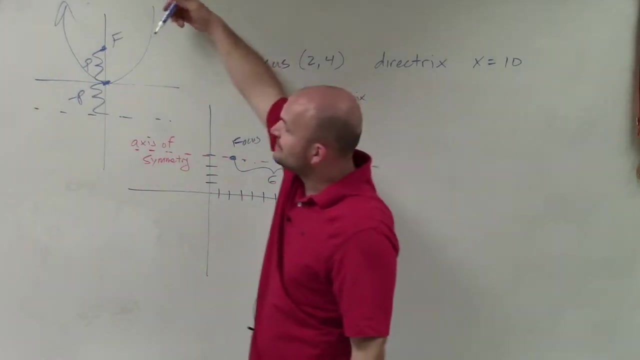 units to the left of my directrix: 1,, 2,, 3, 4.. Perfect, Okay, So now when again determining what the equation is going to be, we need to look at this and say all right, since, remember, the focus is always. 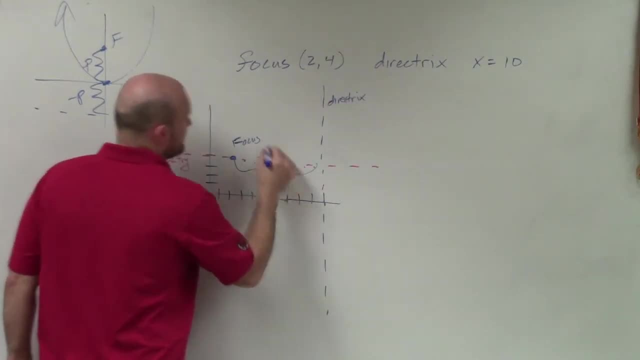 inside of my parabola. So, therefore, my parabola is going to look something like this: All right, Where the distance of P you can see is going to the left, So it's going to be negative. So P equals negative 4. And so where the distance from here is going to be: 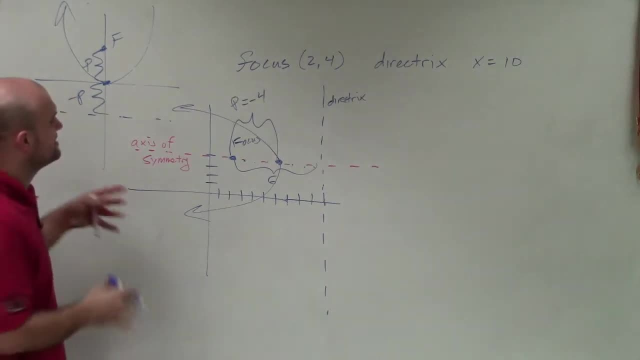 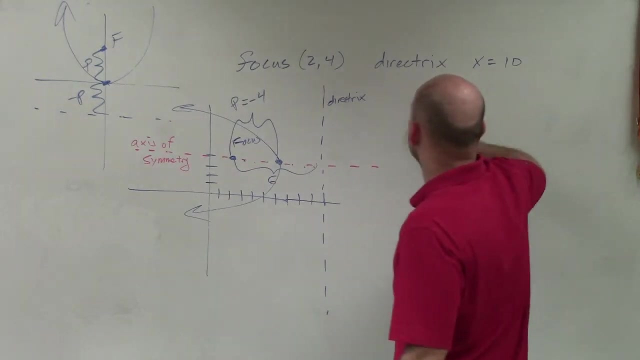 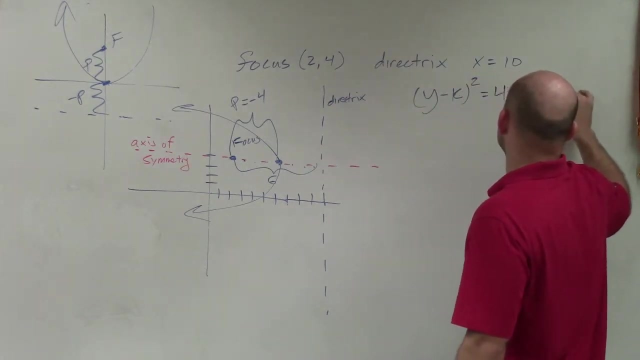 a positive 4 because we're going to the right from the vertex. But what's important is now I know my axis symmetry is horizontal. I'm going to use this equation: X minus- sorry, Y minus K squared equals 4P times X minus H. So what's? 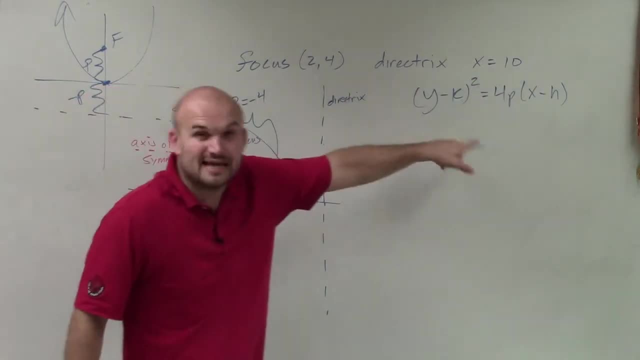 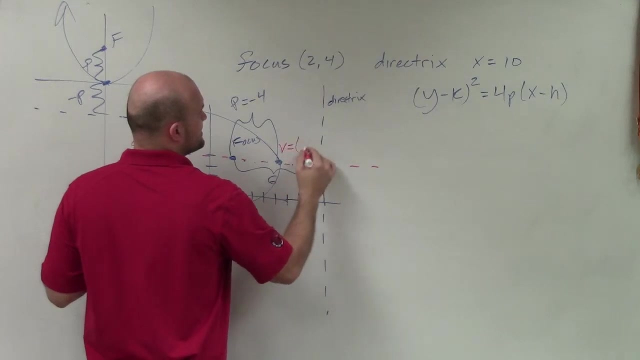 important about this now is now I need to make sure I identify for my H and K which will be my vertex. So I know that it lies on the axis symmetry. So therefore my Y coordinate is still going to be 4.. But now it's going to be 4 over from my focus. So 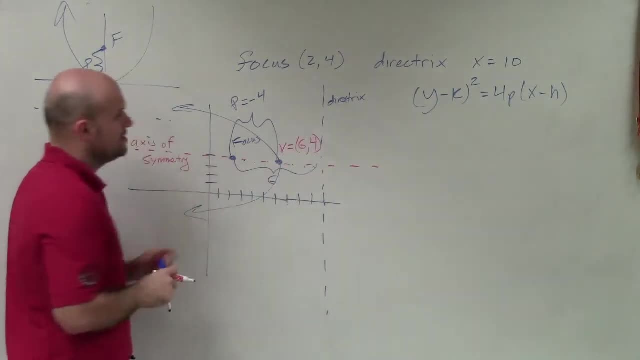 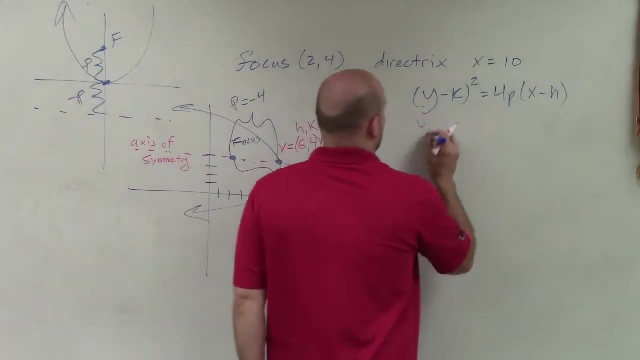 that's going to be 6 comma 4.. So now I can say my vertex is 6 comma 4, which, remember, represents H and K. So now I'm going to plug that in. So I'll say Y minus H, which is: 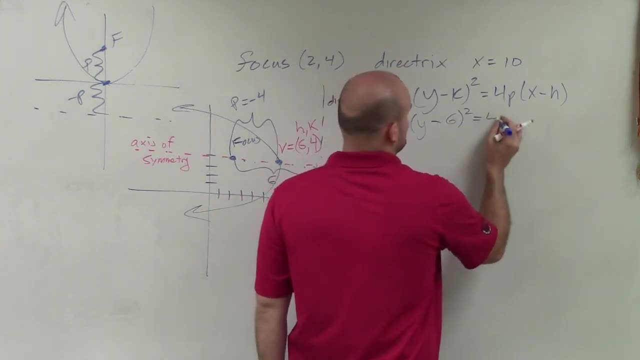 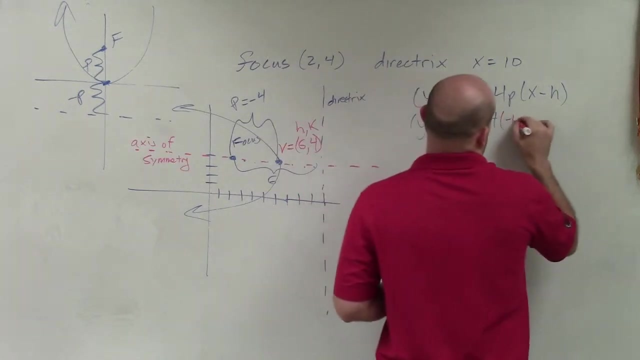 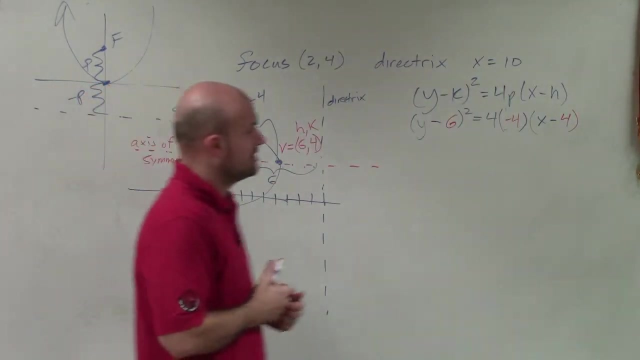 6 squared equals 4 times my P, which in this case is negative 4.. I want to write that in there: Times X minus 4.. Okay, So now what I need to do to write the standard form of the equation is: I need to. 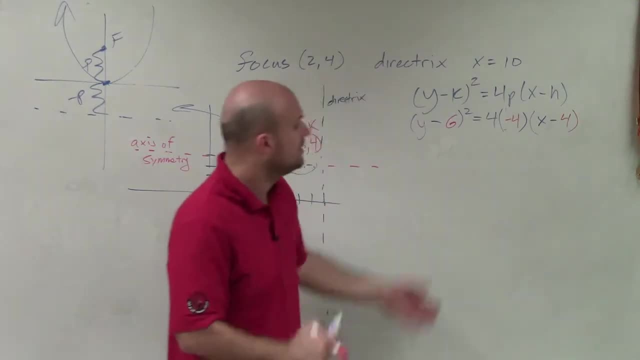 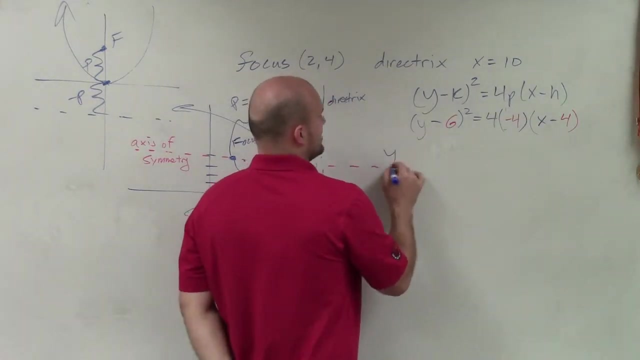 expand my binomial squared, which will produce a perfect square trinomial, as well as apply the distributive property across over here. So Y minus 6 squared, it's going to be Y squared minus 12Y plus 36 equals 4 times negative. 4 is 16.. So negative 16 times X is a negative. 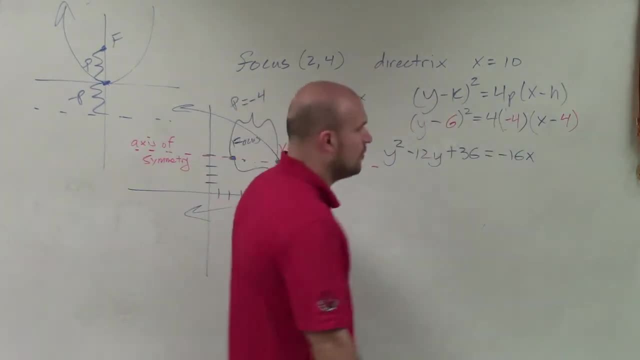 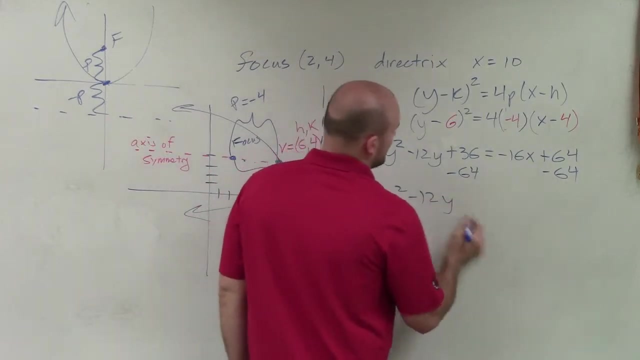 16X And negative 16 times 4 is going to be a positive 64. So now I need to isolate my X, So I'm going to subtract 64 on both sides. So I have Y squared minus 12Y, 36, that's going.